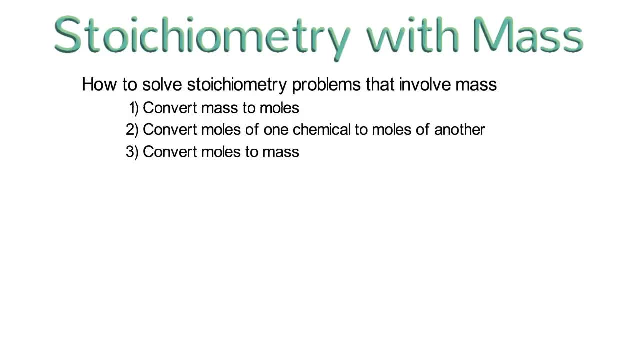 seem like a bit much, but they are necessary because you must be in moles in order to convert from one chemical to another. Let's see how these three steps work for a problem involving food. Suppose that you are a chef at a grilled restaurant and you are also in charge of ordering. 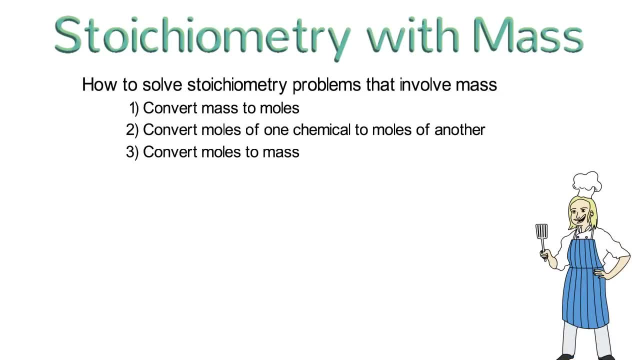 all the ingredients you need. Unfortunately, you are completely out of hotdog buns and your supplier sells everything in pounds. If you have eleven pounds of extra hotdog meat, how many pounds of buns do you need to purchase? Start the problem by writing down the amount of calories you need to convert from one. 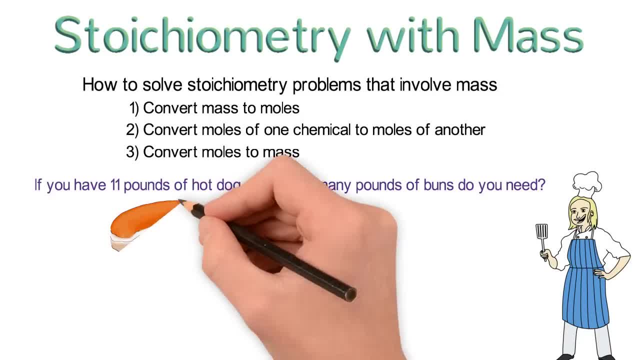 writing down the balanced reaction that is your recipe. One bun and one piece of hot dog meat are needed to make one hot dog. Now, in order to figure out how many buns you want to buy, you need to first calculate the number of hot dogs that you have. 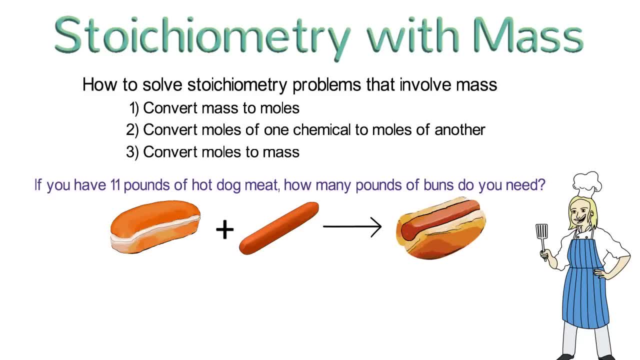 And in order to do that, you need to know how much one hot dog weighs. It's best to write down the individual mass of every reactant and product. One bun weighs 0.1 pounds. One dog weighs 0.125 pounds. 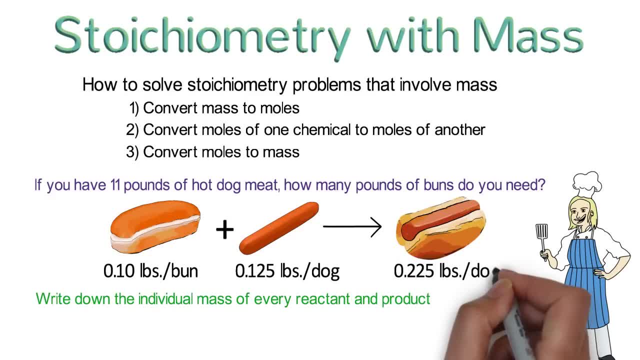 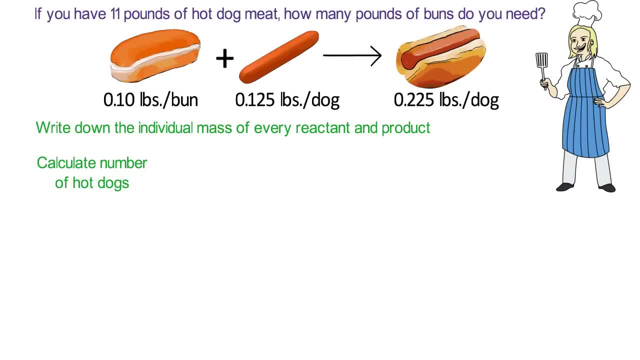 And a hot dog with bun weighs 0.225 pounds. Next we need to calculate the number of hot dogs we have. This is a unit conversion problem, so we first write down the quantity that we know: 11 pounds of hot dogs. 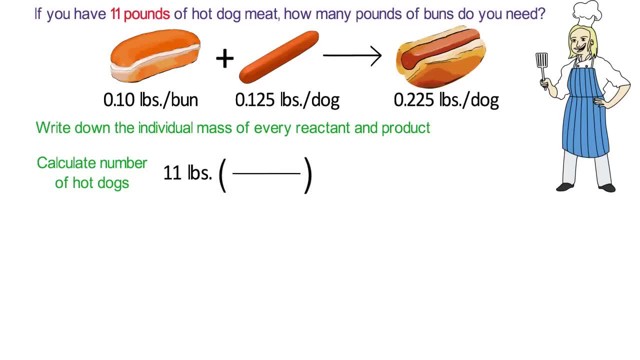 Multiply this by a conversion factor fraction. The weight of one hot dog is our conversion factor. Because we are starting with pounds, we put the 0.125 pounds on the bottom of the fraction And because we are solving for the number of pounds, 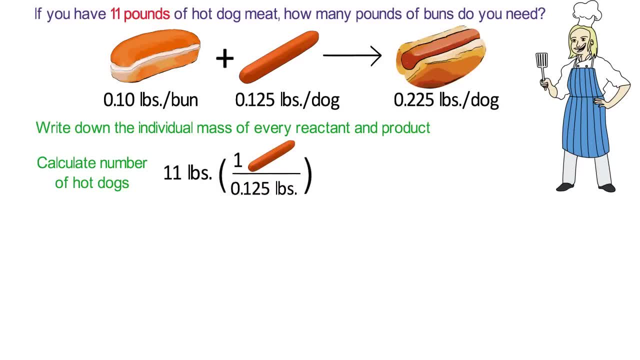 we put one hot dog on top. Remember that our conversion factor fraction is always equal to 1.. Because one hot dog weighs 0.125 pounds, the fraction 1 hot dog over 0.125 pounds is equal to 1.. Now let's do the calculation. 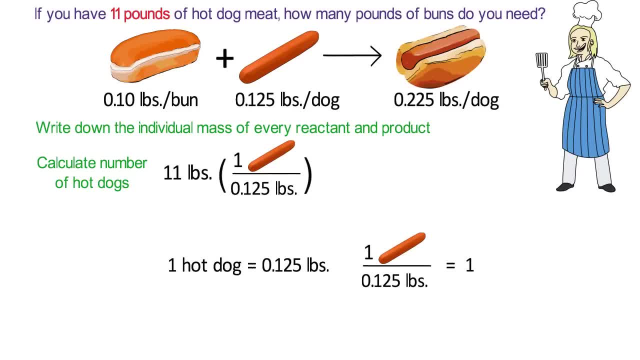 The number of hot dogs is 11 times 1 over 0.125.. Because the 1 is on top, we type in our calculator 11 divided by 0.125, and the answer is 88.. As for the units, pounds on top cancels with pounds on the bottom and we are left with 88 hot dogs. 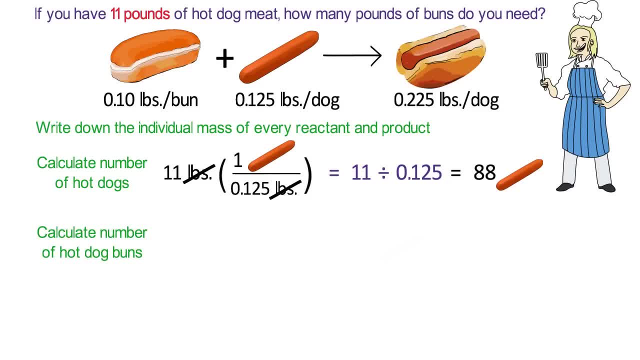 Next we need to calculate the number of hot dog buns we need. This is also a unit conversion problem. so we start by writing down the number. we know: 88 hot dogs. Multiply this by a conversion factor fraction. This time our conversion factor is the balanced reaction or recipe. 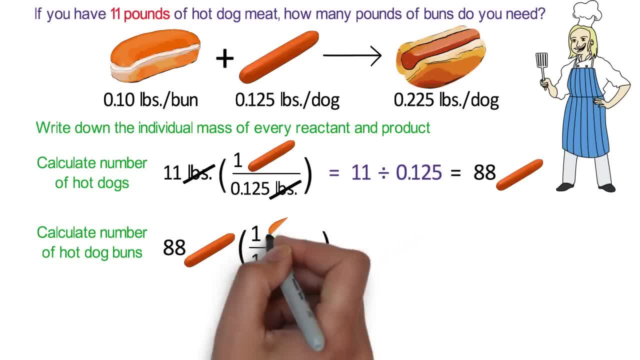 From the recipe we know that one hot dog needs one bun. Hot dogs on the top need one bun. Buns on the top and bottom cancel and our answer is 88 buns. We need 88 buns, but our supplier wants to know the weight of buns we need. 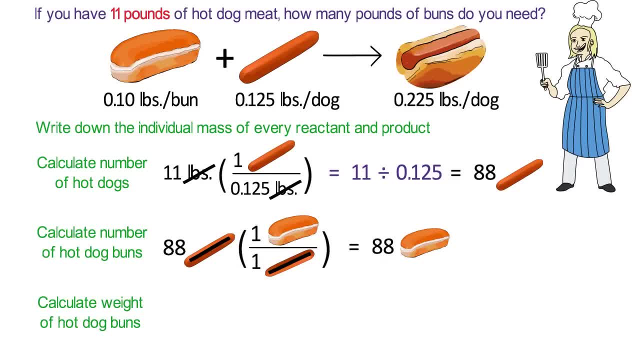 so we are going to convert this back into pounds. The number we know is 88 buns and we multiply this by a conversion factor fraction. The weight of a bun is our conversion factor, Because we are starting with number of buns. we put one bun on the bottom of the fraction and 0.1 pounds on the top. 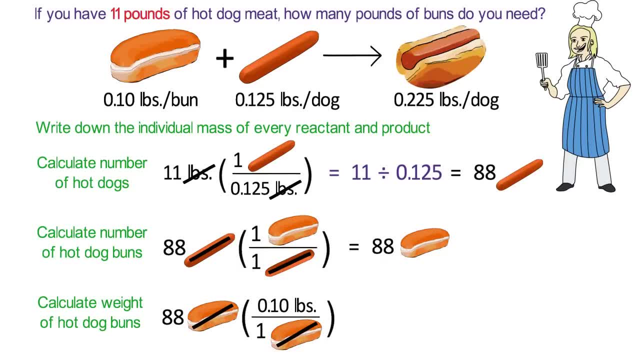 Buns on the top and bottom cancel out to give us as our final units For the calculation the 1 in the fraction is on the bottom. so in your calculator type, 88 times 0.1, which gives us our final answer of 8.8 pounds of buns. 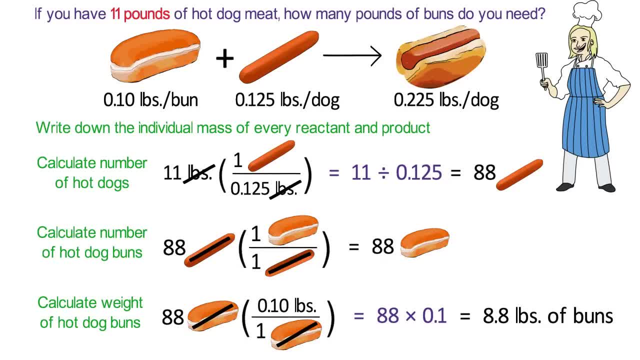 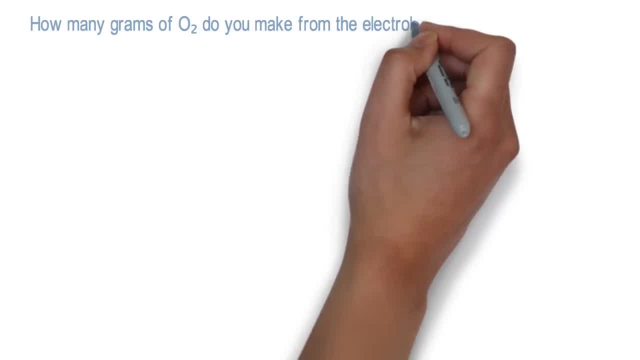 This is the typical three-step calculation for most stoichiometry problems. Let's try this now with a chemical reaction. How many grams of oxygen do you make from the electrolysis of 100 grams of water? The electrolysis of water is a decomposition reaction. 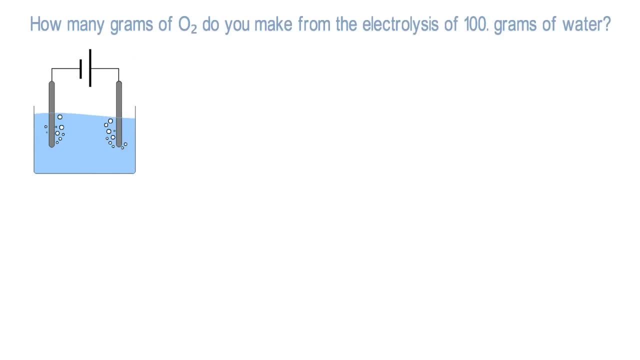 in which water breaks down into its elements oxygen and hydrogen. Because the reaction needs a continuous supply of electricity, it is an endothermic reaction. The first thing that we need to do to solve any stoichiometry problem is to write down the balanced reaction. 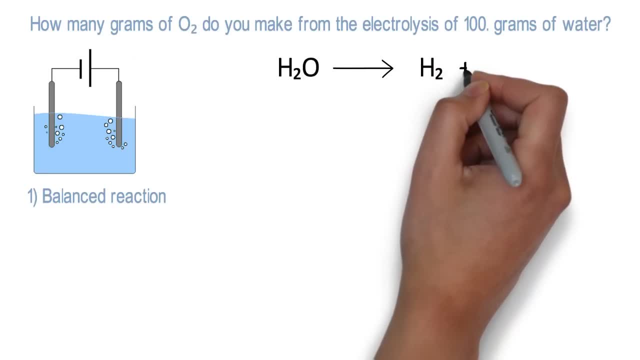 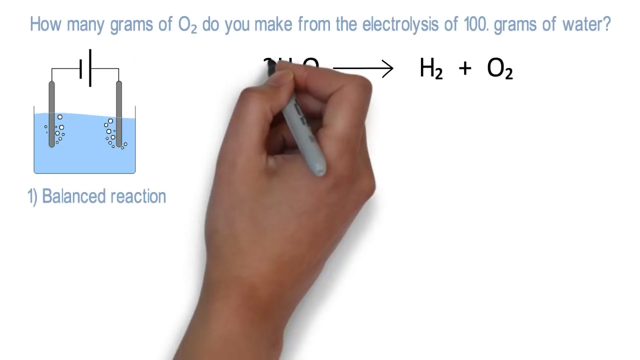 H2O breaks down to form H2 and O2.. Both hydrogen and oxygen are diatomic elements. Pause the video and check this reaction to see if it is balanced or not. The oxygen is not balanced With 1 on the left and 2 on the right, so we put a 2 in front of H2O. 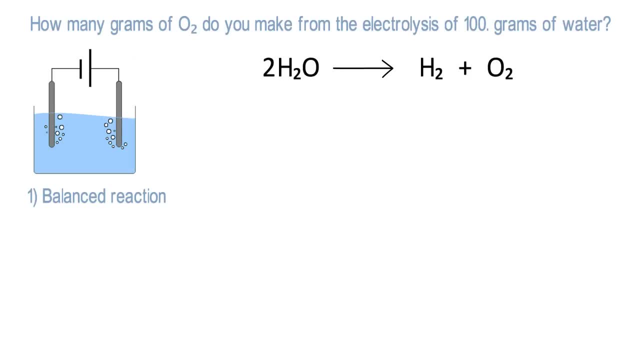 That now makes 4 hydrogens on the left. so we need to put a 2 in front of H2.. The reaction is now balanced. Step 2. Calculate the molar masses of each chemical in the reaction. To calculate the molar mass of water we add together the molar masses of all the atoms in water. 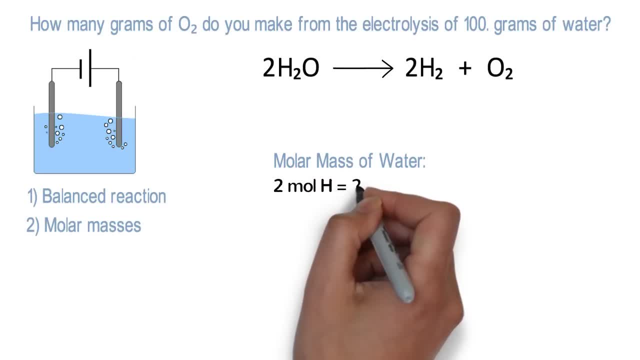 Since there are 2 hydrogens in every water molecule, we multiply 2 times 1.0.. To get 2.016.. There is only 1 oxygen. so that is simply 1 times 16, which is 16.. 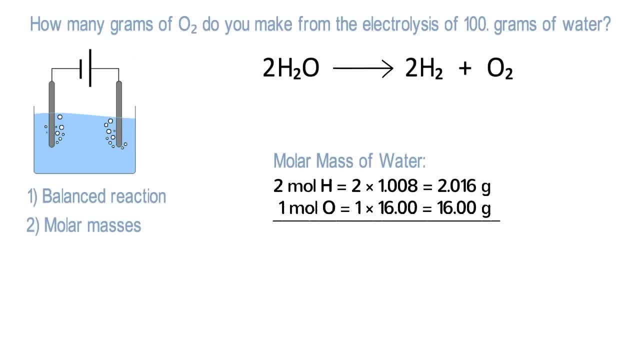 Next add 2.016 and 16 to get a total mass of 18.02.. In other words, 1 mole of water has a mass of 18.02 grams. Notice that the big 2 in front of H2O in the balanced equation did not appear in our calculation of the molar mass of water. 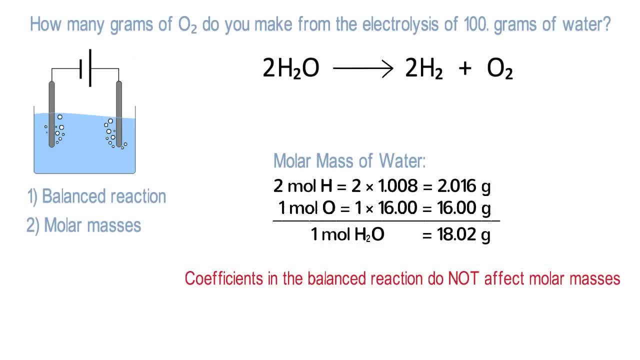 The coefficients in the balanced reaction do not affect the molar masses of any chemical, because the molar mass is the mass of only 1 mole of that substance. Go ahead and calculate the molar mass of every chemical in the reaction and write them below each chemical. 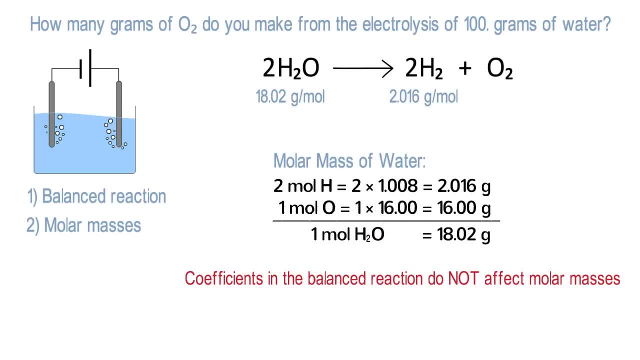 Hydrogen's molar mass is 2.016 grams per mole and oxygen's molar mass is 32 grams per mole. Step 3. Convert the mass of your known quantity to moles. Reread the question. What is the known quantity? 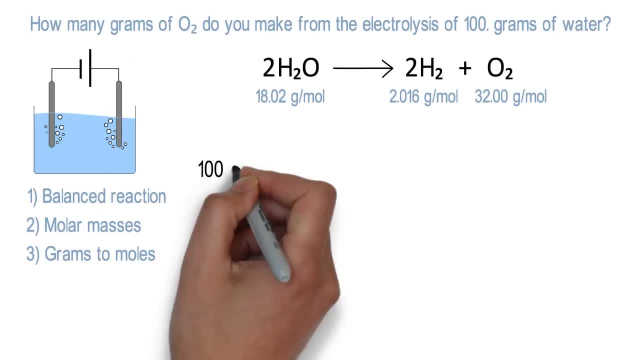 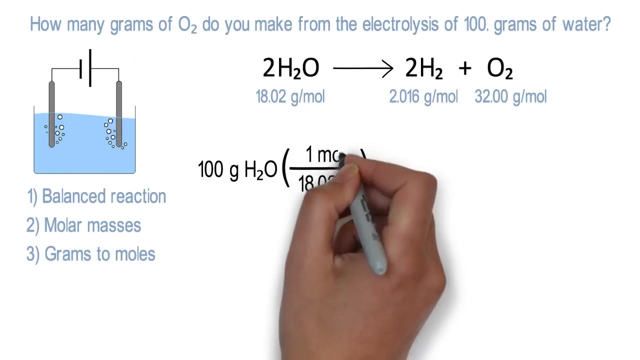 Write 100 grams of water. Write this down first. To convert this to moles, multiply it by a fraction. The molar mass of water is the conversion factor. Because we started with grams, we write 18.02 grams on the bottom and 1 mole on the top. 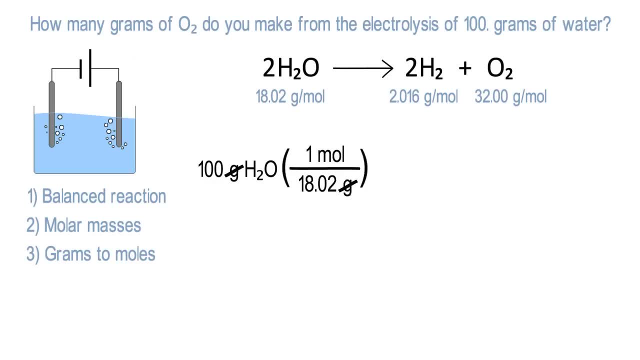 Grams on the top and bottom. cancel out because the 1 is on the top of the fraction in your calculator, type 100 divided by 18.02.. The answer works out to be 5.55 moles of water. Step 4. Convert the moles of water to moles of whatever you are solving for. 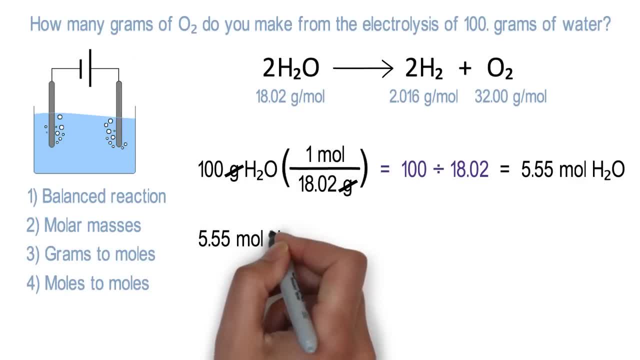 Write down the answer from the previous step- 5.55 moles of water- and multiply this by a fraction. This time the balanced equation is our conversion factor. The coefficients in the balanced equation tell us the ratio of the chemicals in the reaction. 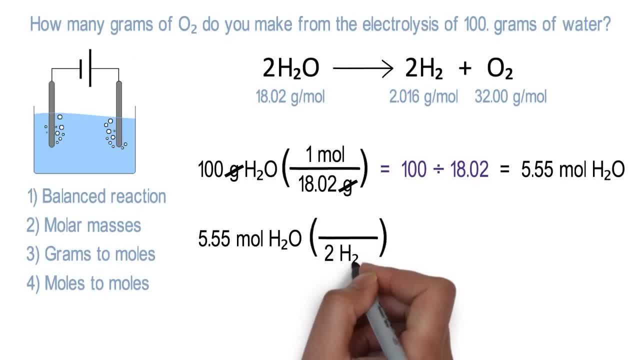 Because we started with moles of H2O. write 2H2O on the bottom. Because we want to convert this to oxygen. write 102 on the top. Remember that if there is no number in front of the chemical, the coefficient is really 1.. 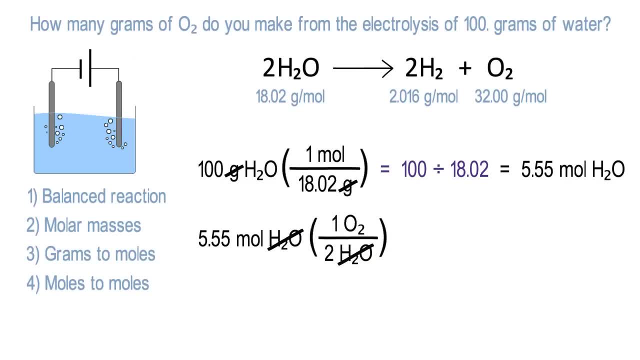 H2O on the top and bottom. cancel out because the 1 is on the top of the fraction in your calculator type, 5.55 divided by 2, which works out to be 2.775 moles of oxygen. The last step is to convert the moles of oxygen to grams. 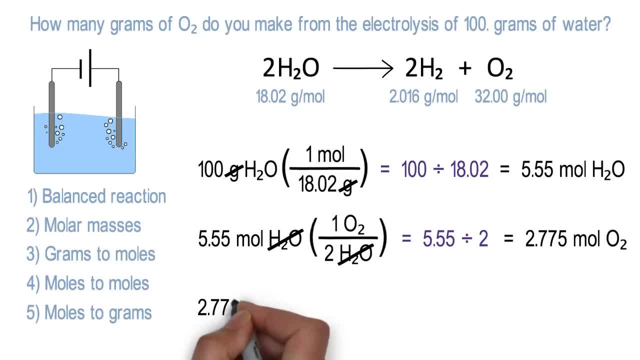 Write down the answer from the previous step: 2.775 moles of oxygen. Write down the answer from the previous step and multiply this by a fraction. The molar mass of O2 is our conversion factor Because we started with moles. 1 mole goes on the bottom and 32 grams goes on the top. 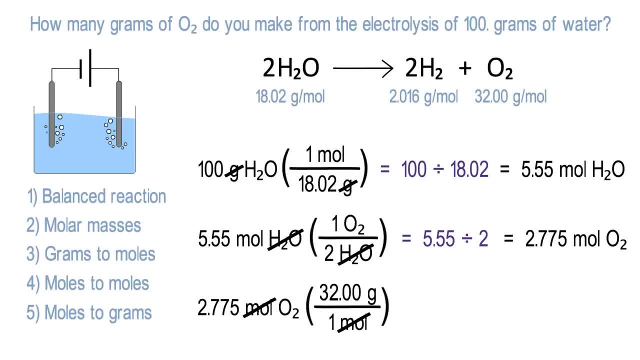 Moles in the top and bottom cancel out because the 1 is on the bottom of the fraction in your calculator type, 2.775 times 32, which works out to be 88.8 grams of oxygen. This is our final answer to the problem, but we should check to see if it makes sense. 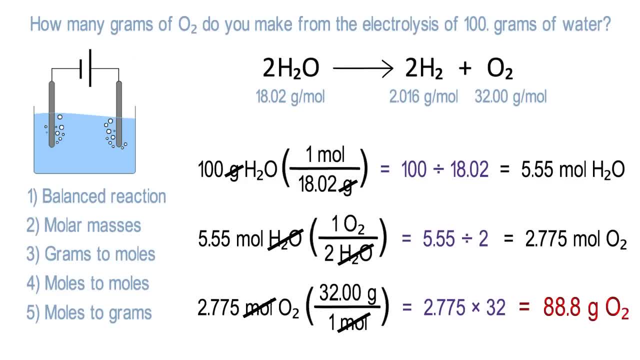 Because water is decomposing into two products, we expect our answer to be less than 100, which it is. Because oxygen is much heavier than hydrogen. most of the mass should go into O2 rather than H2, so our answer should be greater than 50, which it also is. Therefore, 88.8 grams is quite reasonable. 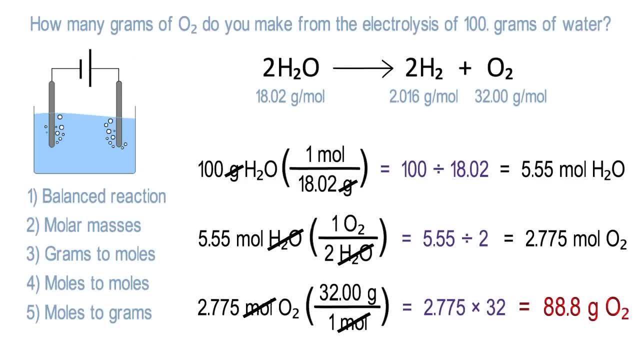 Remember to follow these steps when solving a stoichiometry problem that involves mass, and the only way to get good at it is to practice, practice, practice. Thanks for watching. If this video helped you out at all, please give me a thumbs up. 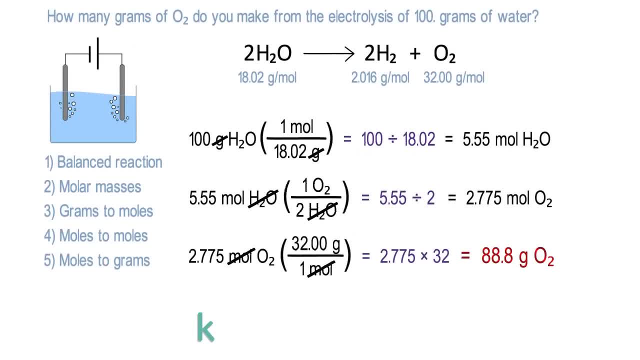 It means a lot to me. Feel free to also share any comments or questions you have below. subscribe to my channel or check me out at ketzbookcom.